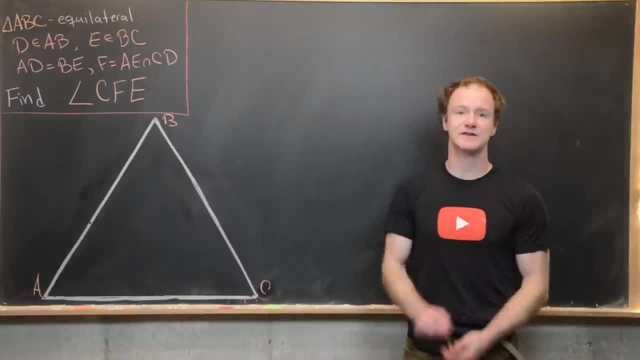 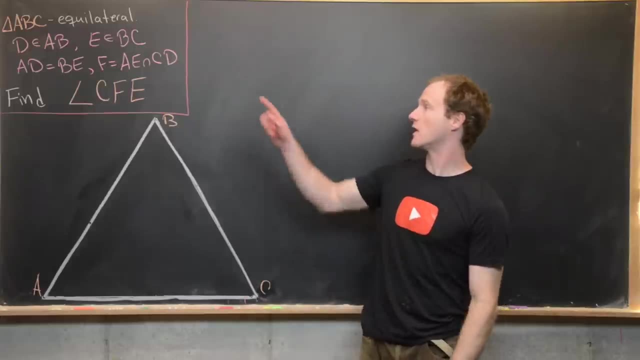 you're interested in that, And so our setup goes like this: We've got an equilateral triangle- A, B, C- And then next we have a point D on the line segment AB and a point E on the line segment BC. 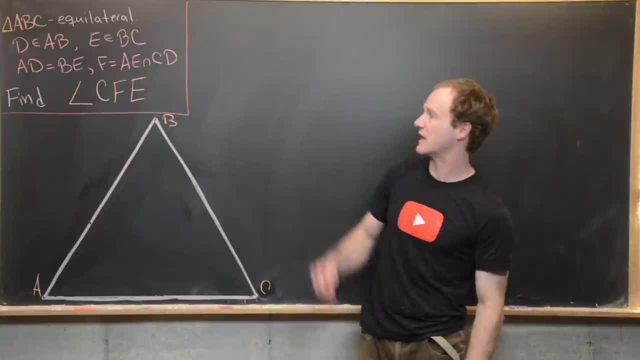 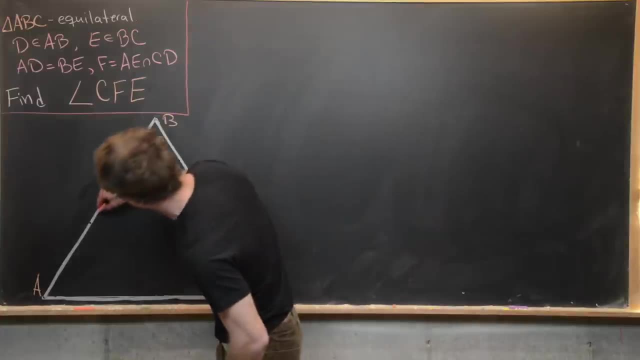 And they are arranged in a way so that the line segment AD and the line segment BE are the same length. So that means, I could maybe put D right here, and then I could put E right here, And so in other words, here we've got AD, which I'll put in pink like this: 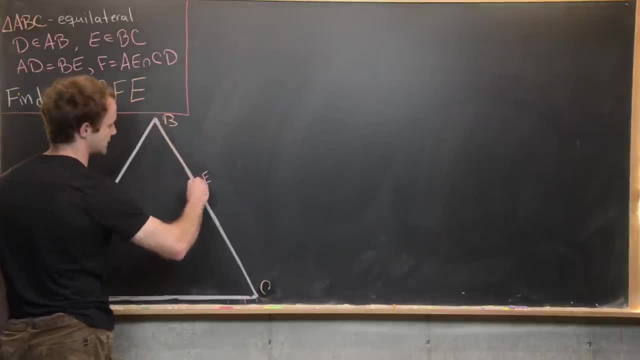 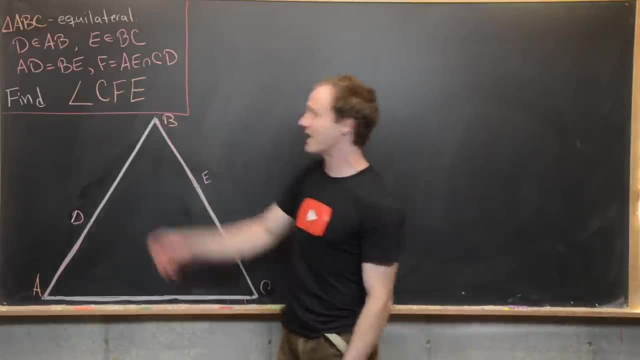 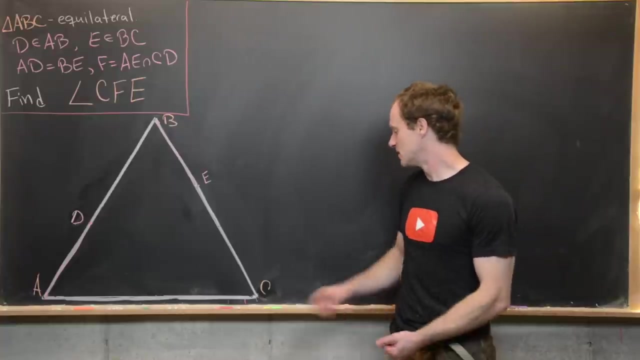 is equal to BE, which I'll also put in pink like this. Okay, So that's our first setup, And then next we want to let F be the intersection of these line segments, AE with CD. So let's maybe put those line segments on the board. So AE. So that's going to. 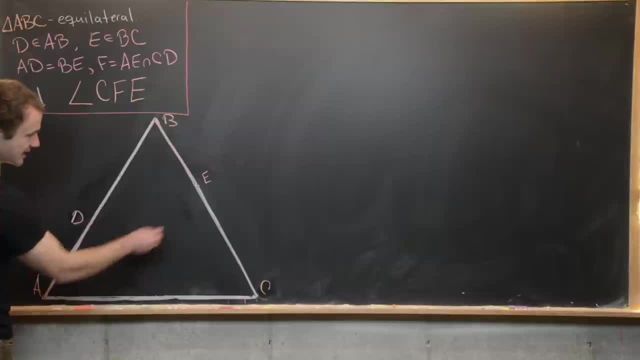 be like from this vertex of the triangle to this point right here which we added. So let's see, that's something like this. And then we want CD, So that would be kind of that, its companion over Here, So that would be something like this: Good, And then this point here at the intersection is: 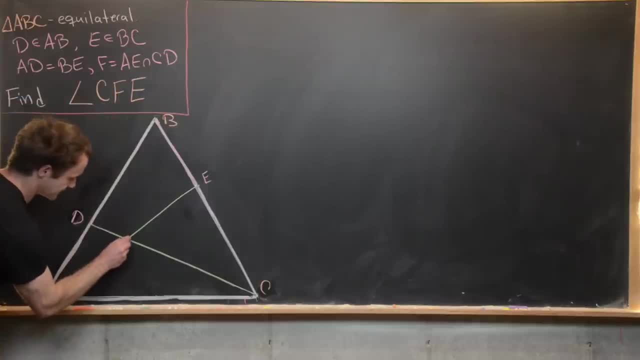 the point that we're going to call F, So that would be this point right here. And then our goal is to find the angle measure of CFE. So maybe we'll give this thing a name, Let's maybe call this angle theta- And so our goal is to find that angle measure theta. So we're going to 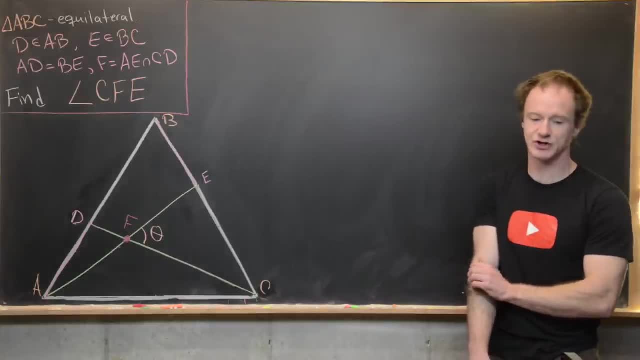 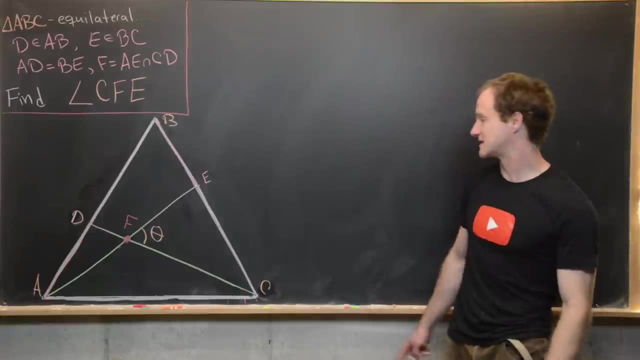 focus on two small triangles that make up this picture, And those two small triangles will be triangle ABE and also triangle CAD, And actually those triangles seem to be congruent, And so let's see if we can prove that carefully. So I first want to notice that AB, that line segment. 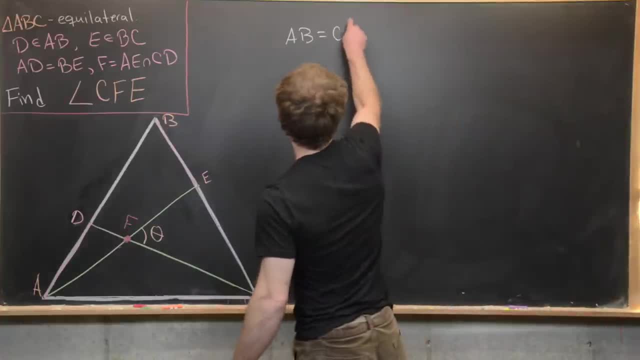 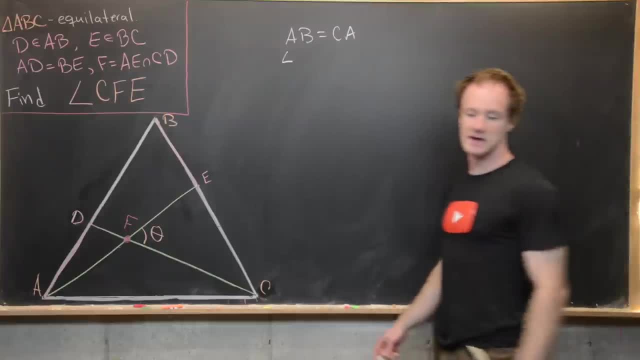 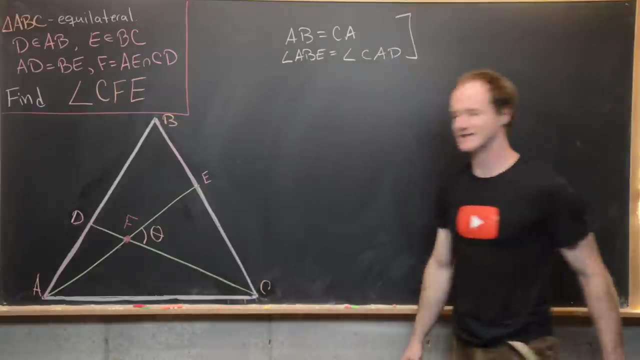 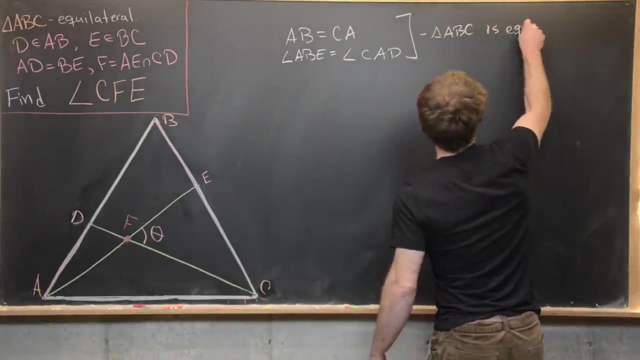 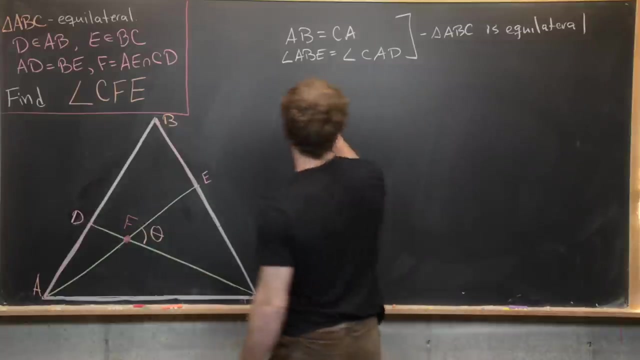 furthermore, we have angle measure: ABE is equal to angle measure CAD. Okay So, and both of those are equal to 60 degrees. And again, these two facts come from the fact that triangle ABC is equilateral. Great, Now we can apply our given fact, which is that AD equals BE. So let's write. 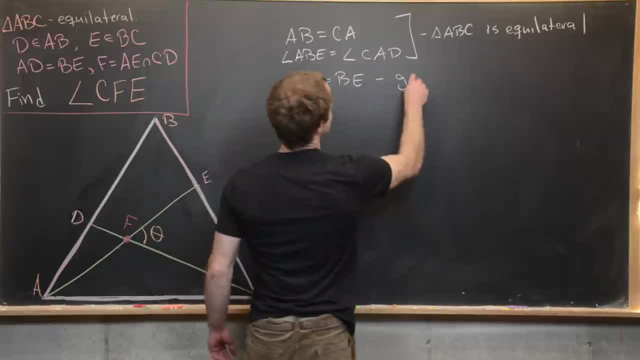 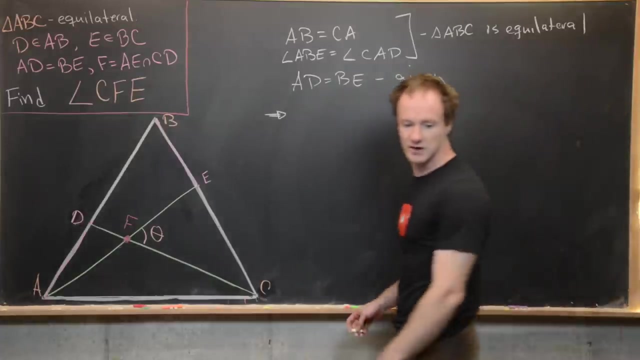 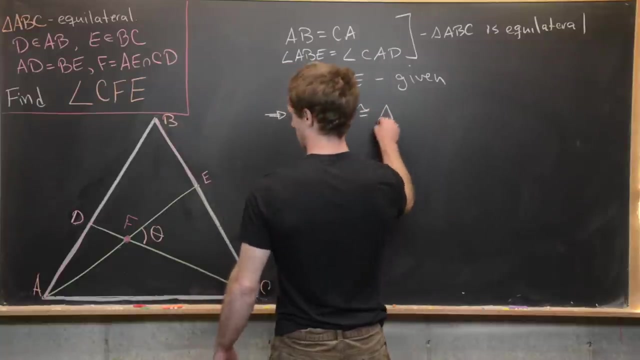 that here AD equals BE, And so that's given in the problem. And so these three things together, side, angle, side, imply that those two triangles that seem to be congruent are actually congruent. So in other words, we have triangle. ABE is congruent to triangle. let's see what it is CAD. Now we can. 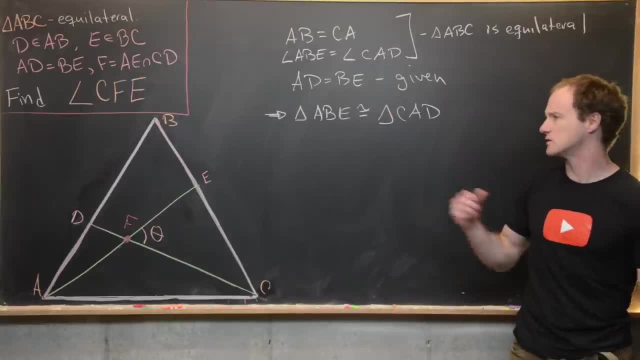 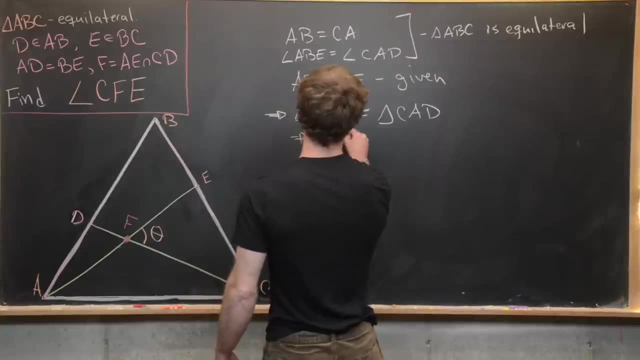 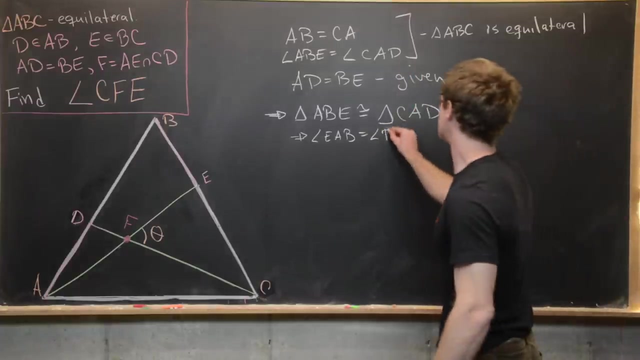 do that by taking some more information out of this. So we know that all of the component angles and sides of these two triangles have to be congruent. In particular, this tells us that angle EAB is equal to, in measure to triangle DCA. So let's maybe put those on the board in. 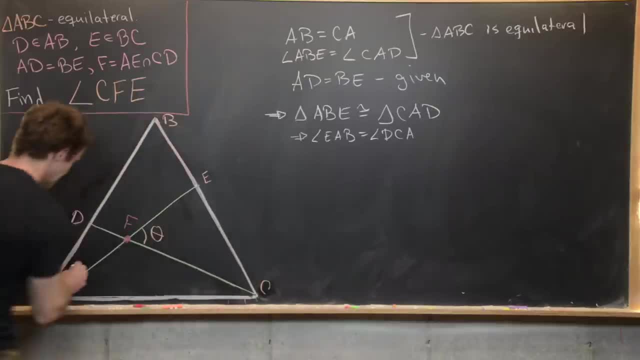 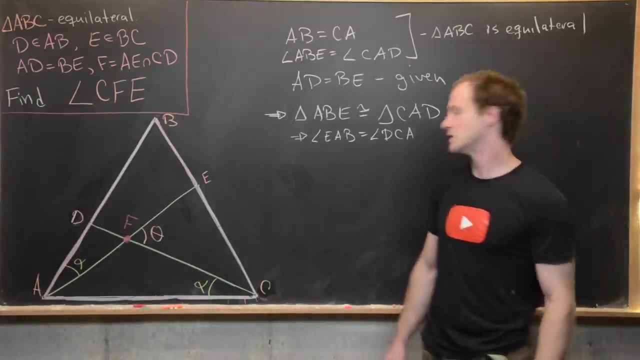 yellow. So EAB, that's going to be like this angle right here. So maybe I'll name that alpha, And then d, c, a. so that's going to be down here. that is also angle alpha, and now we're ready to start finishing this off. so notice that we know that this entire angle here, d a c, is going to be 60. 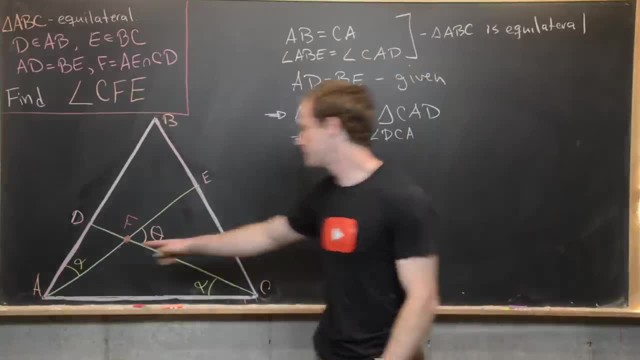 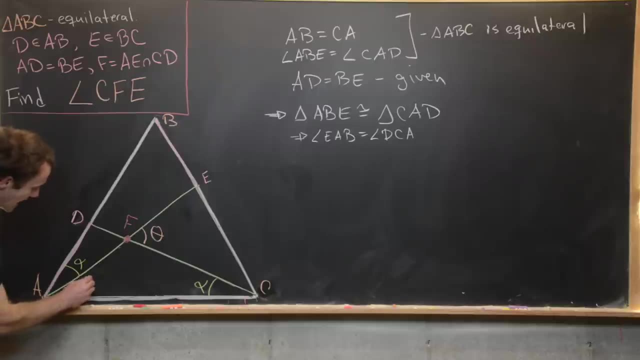 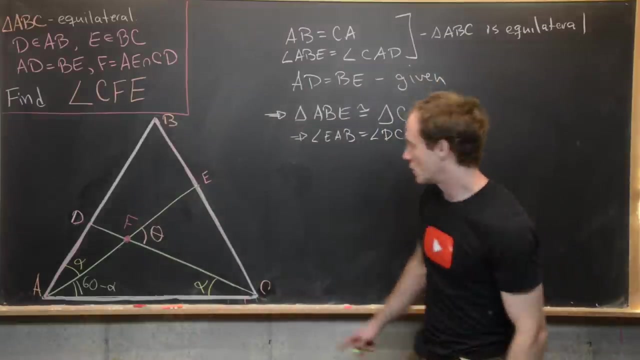 degrees. that's because this whole triangle is equilateral. this portion of the angle has measure alpha, but that's going to tell us that this portion of the angle has measurement 60 minus alpha. okay, and then next we know that the sum of the angles of a triangle add up to 180. 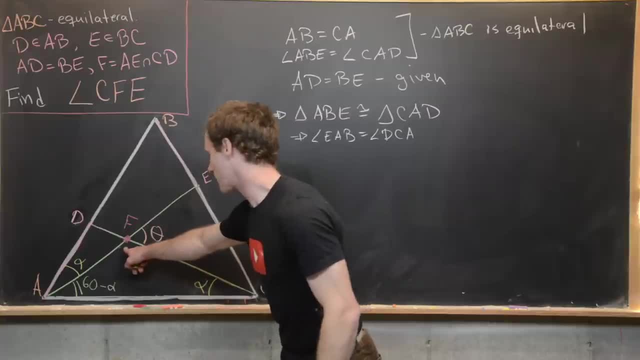 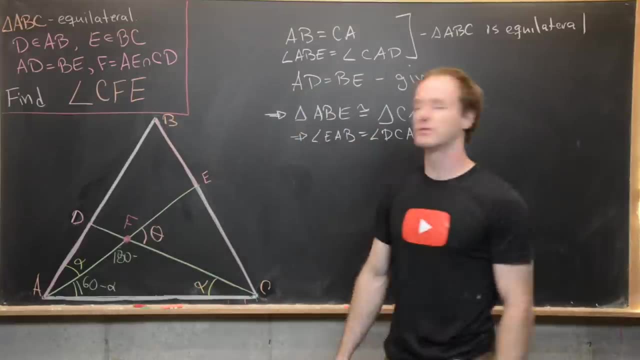 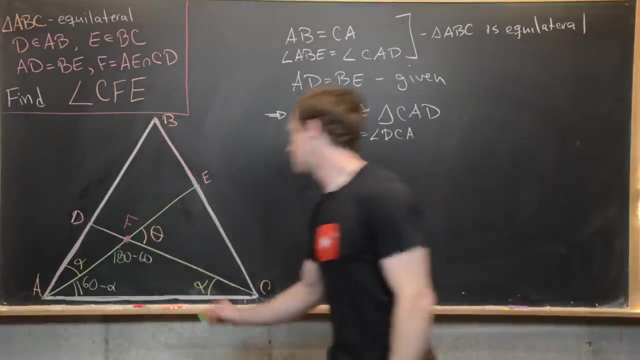 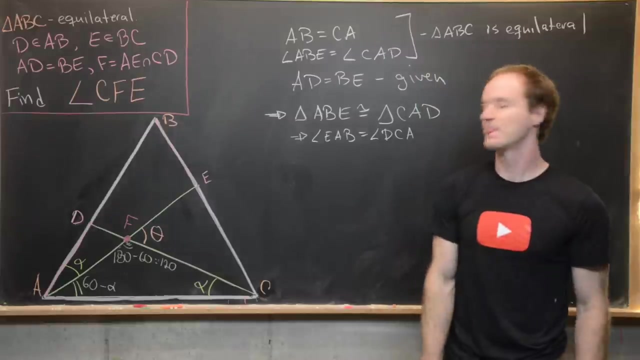 so that means that this number right here is going to be 180 minus 60 minus alpha plus alpha, but 60 minus alpha plus alpha is just 60. so we get that right there. so that's going to make this 120.. so that's this angle measurement right here. and then finally, because this makes a straight line,